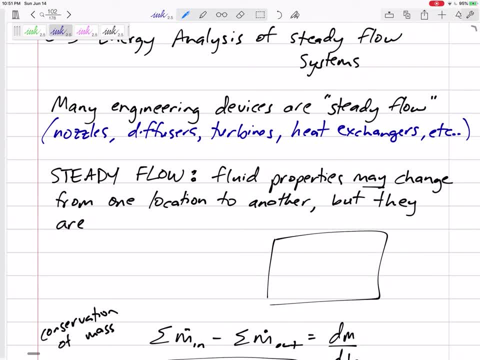 exchangers. Steady flow just means that the properties may change from one location to another. So at the inlet might have different properties than the outlet, but they are steady in time. They are steady in time, They are constant in time, They don't start at one. 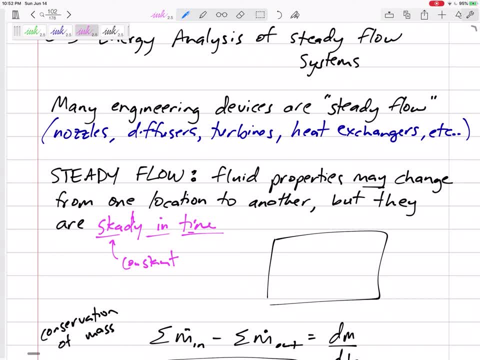 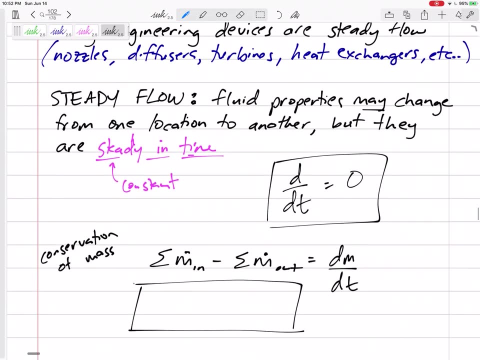 value and then at the end, after one hour, they are a different value. Their derivatives with respect to time would be zero. If they're constant in time, then their derivative ddts will be equal to zero. They're not changing in time, right? They're not changing in time. So our conservation? 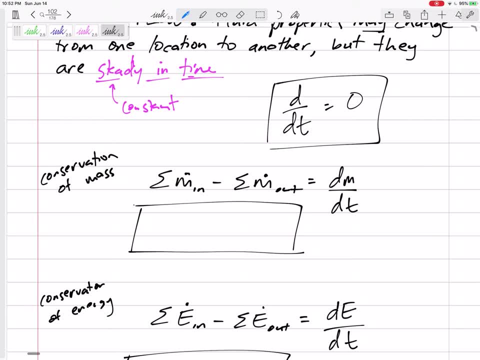 of mass. all the mass coming in minus all the mass going out, equals the change in mass per time. The change in mass per time is zero for steady flow devices. Let me kind of make it up: Zero for steady flow devices. So now, m in minus m out equals zero, Do you mind? 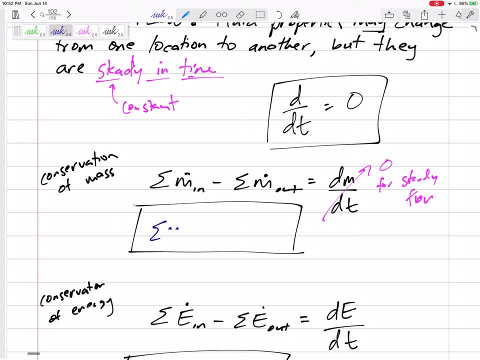 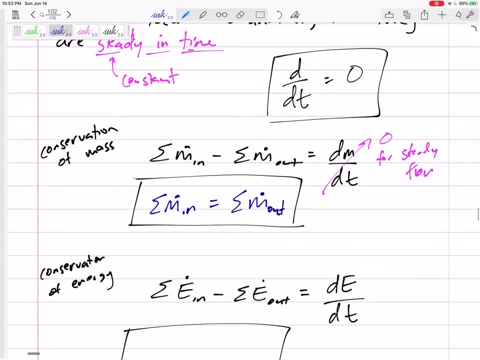 if I take that m out to the other side of the equation. So now the sum of all the m in equals the sum of all the m out for steady flow devices. If you write that equation on your formula sheet, on your note card, make a note: hey, steady flow devices. Or you can. 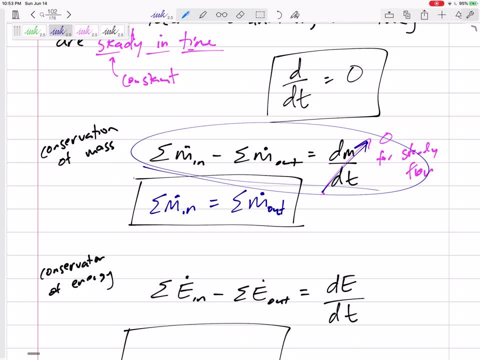 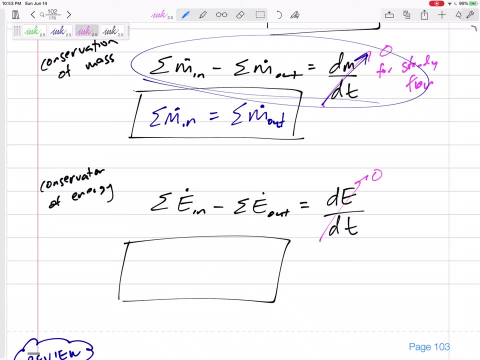 start here, know it's steady flow. and then you've got that equation. Same thing with energy, Same thing with conservation of energy. The change in energy, The change in energy over time, all right, not the change in energy from the inlet to the outlet, but the change in. 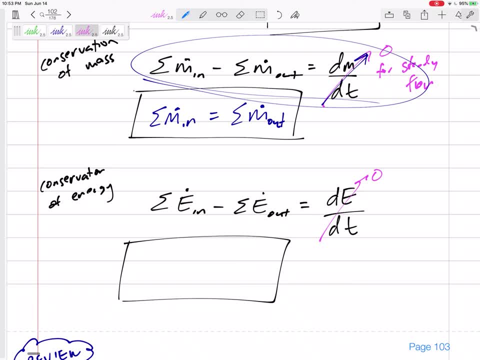 energy after an hour, after two hours, after four hours is zero for steady flow devices. And so do you mind if I take that energy to the other side of the equation. The sum of all the energy in equals the sum of all the energy out, The sum of all the energy in. 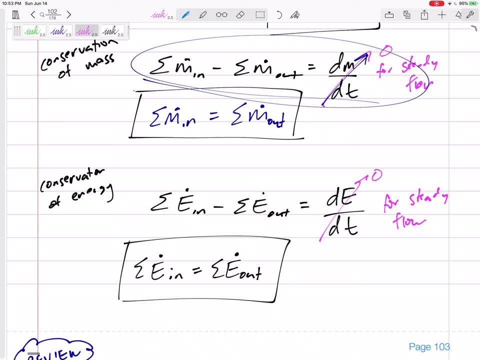 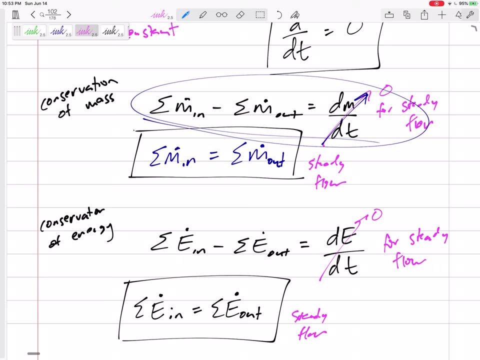 equals sum of all the energy out for steady flow devices. I can't emphasize that. enough Steady flow, steady flow. But we are going to look at a lot of steady flow devices. A lot of our devices are steady flow devices. The way that I think about it is this: if it's not collecting mass, 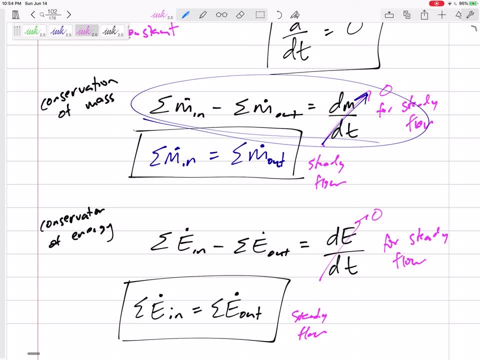 if it's not filling up with mass. if it's not, you know, if the mass is not changing inside of our control volume, then it's a steady flow device. All right, let's look back at this page. This page was from chapter 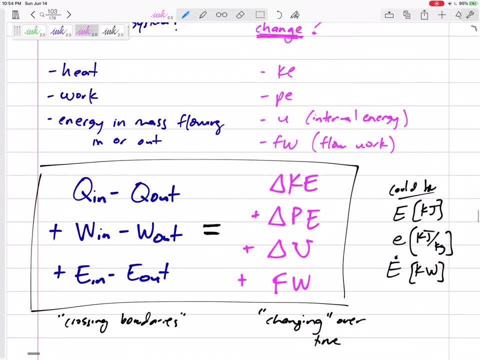 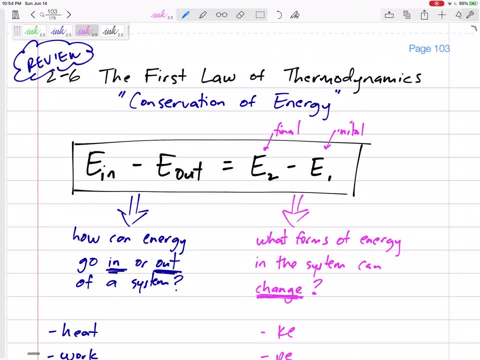 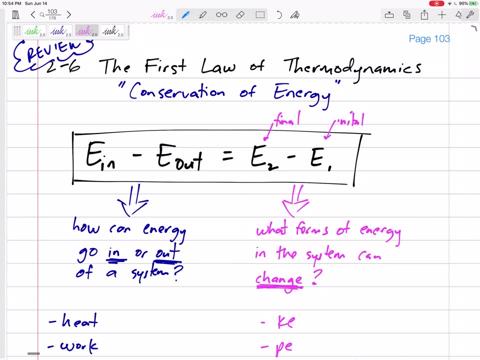 two- This is like the third time I've put it in here in our notes. It's that important right: Conservation of energy. The left-hand side are inlets and outlets. The right-hand side is starting and ending, final and initial in time. Okay, Now these could be capital E's. These, these could be. 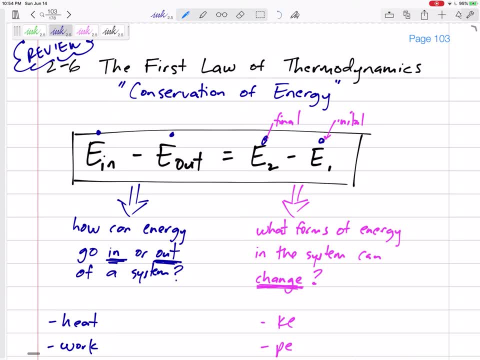 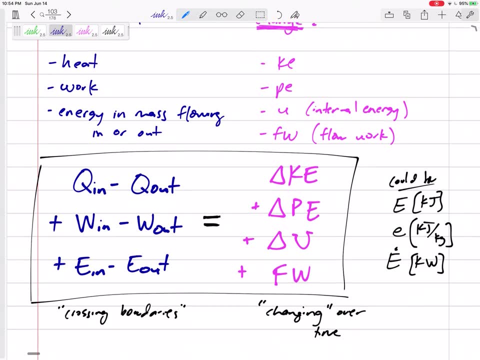 E dots. right, These could be lowercase E's, But for steady flow devices. for steady flow devices, everything on the right-hand side of our equation is going to be zero, And so all we're doing is is, you know, adding up the heat. 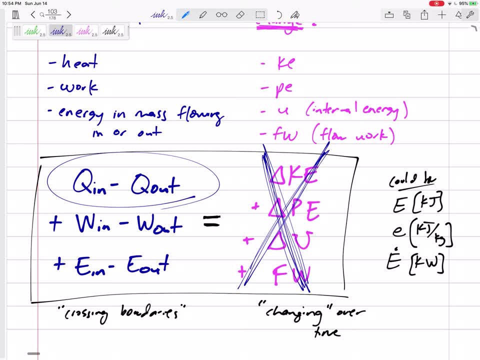 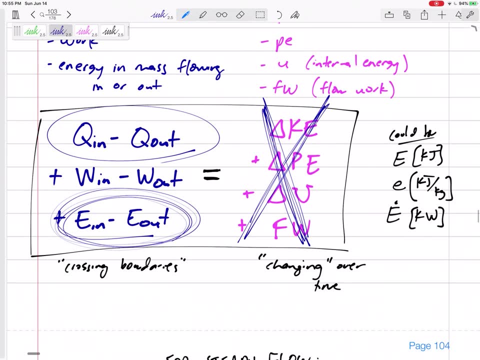 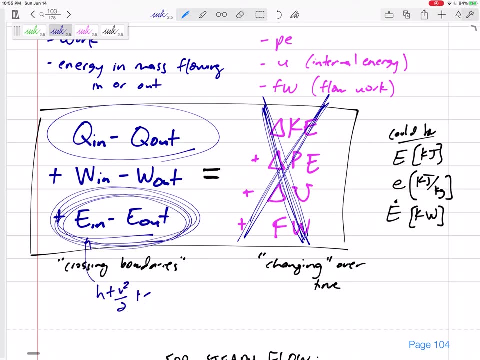 transfer in and out, adding up the work in and out. Now, this is what we haven't had before: the energy in the fluid. This is energy in the fluid right. This is energy in the fluid. This is H V squared over two GZ- H V squared over two GZ. Okay, So let's, let's, let's write this: 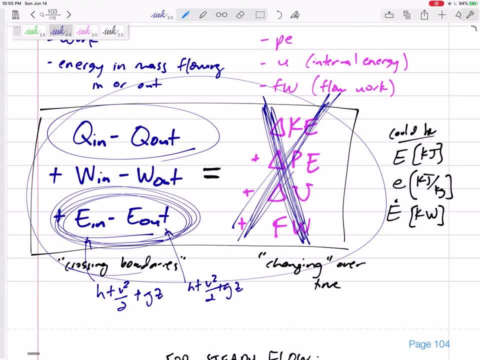 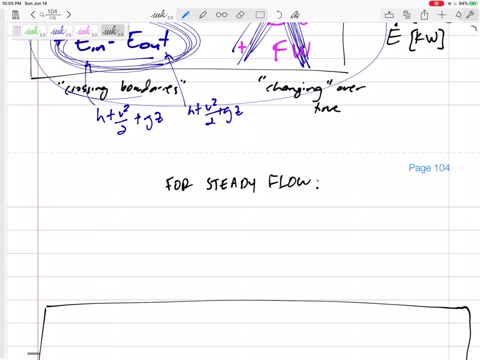 equation right here setting this to be equal to zero. Let's write that equation here, All right. So for steady flow devices, Q in minus, Q out, Q in minus work out, All right. Let's see if, if we want these as like power, like as per unit time. 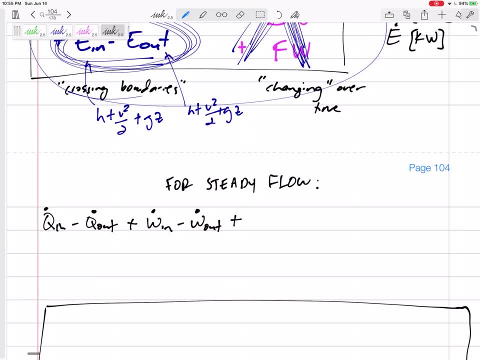 then this E right here would be: M dot theta in minus M dot theta out out equals zero. And aren't you glad that that right-hand side, very quickly, that right-hand side of our equation is is zero. So don't have to worry about the change in time. 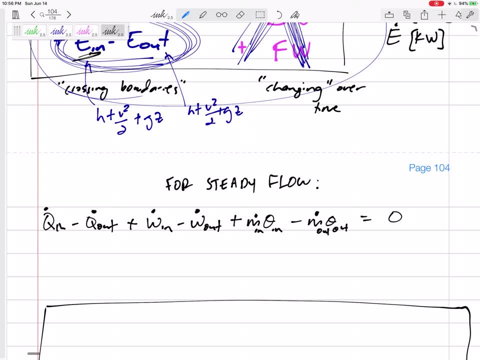 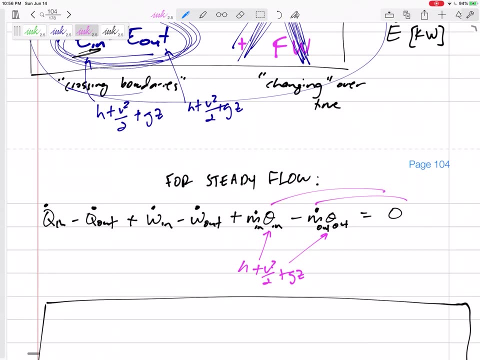 Now, after we're, we're going to get to unsteady flow, but right now that right-hand side of our equation is zero. These thetas are H plus V squared over two plus GZ. H plus V squared over two plus GZ. So so do you mind if I go ahead and take those to the right-hand side of our equation? 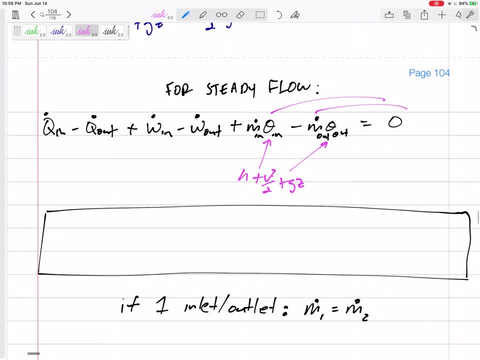 I'm going to leave the Q's and W's on the left-hand side of our equation, but I'm going to take the um energy in the flowing fluid to the right-hand side of our equation. So I'm going to take the energy in the flowing fluid to the right-hand side of our equation, So it becomes Q and W. 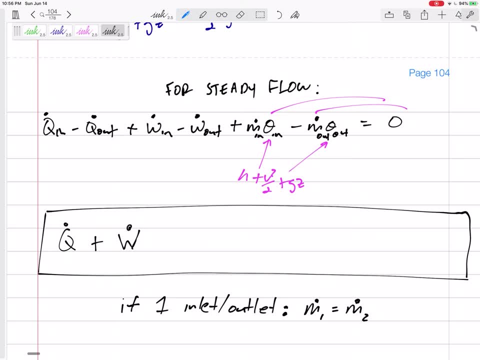 I'm just going to put Q plus W, but but you know that N means positive and out means negative. equals M dot. Let's see, when we subtract this over, this term becomes positive, this term becomes negative. So let's do out first M dot, out H out V squared over two out GZ out. So that's. 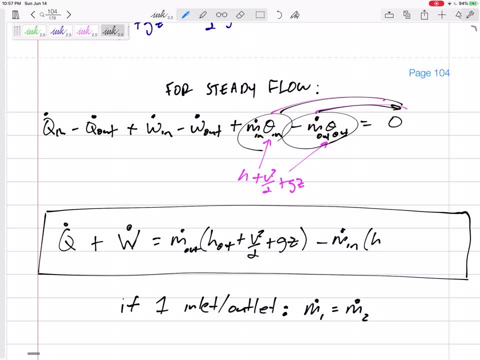 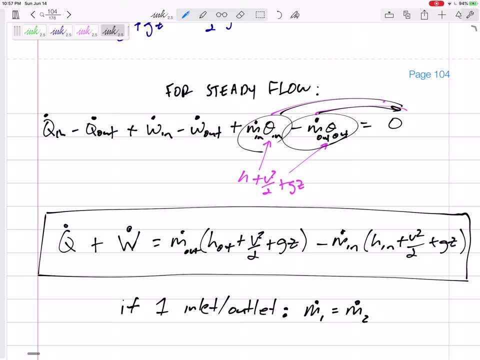 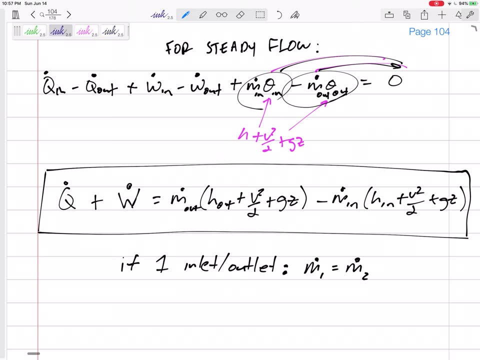 minus M dot in H in V squared over two in GZ in All right, That equation right there. if you only write one equation down on your formula sheet, write that one down Now. make a note. this is for steady flow, but that is our conservation of energy. equation for steady flow: The left-hand. 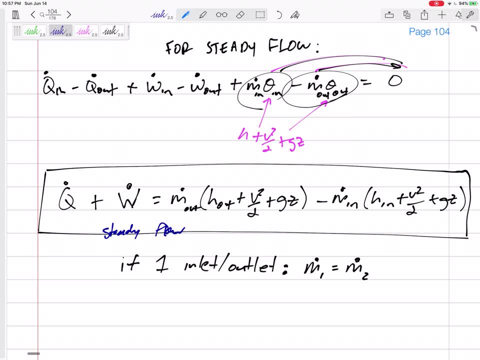 side is heat transfer. crossing the boundary. Left-hand side is work. crossing the boundary. The right-hand side is energy in the inlet and energy in the outlet. All right, Energy in the inlet and energy of the outlet. Okay, So that's our, that's our main equation. I might just start with that one every time. 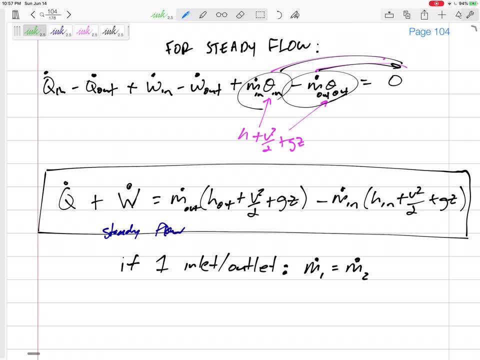 start with that one every time: Um, and it simplifies. you know, maybe there's no potential energy, Um, maybe there's no kinetic energy. here We're going to simplify it a little bit by saying: uh, there, if there's one. 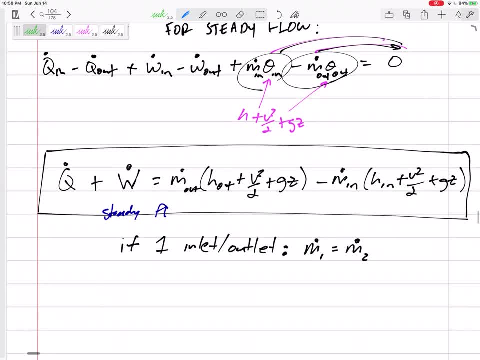 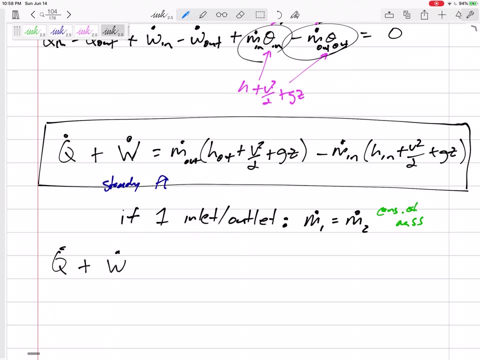 inlet and one outlet, then conservation of mass would tell us: M dot one has to equal M dot two. So we could kind of factor that out And we've got this equation: Q and W equals just one M dot. And then, and then like: 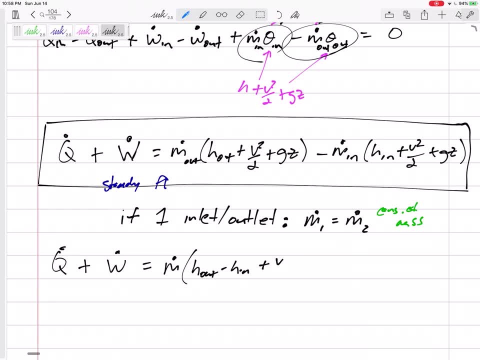 let's go ahead and do the H out minus H in V, squared over two out minus V squared over two in G Z. you know change in in Z, So we can kind of, you know, group the potential energy together. 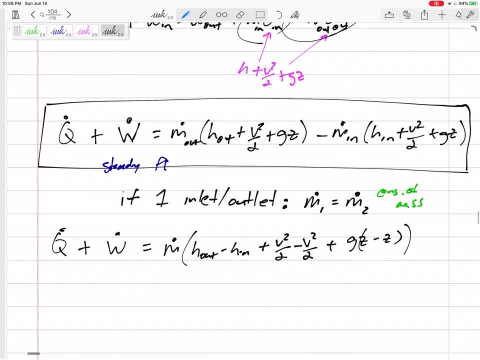 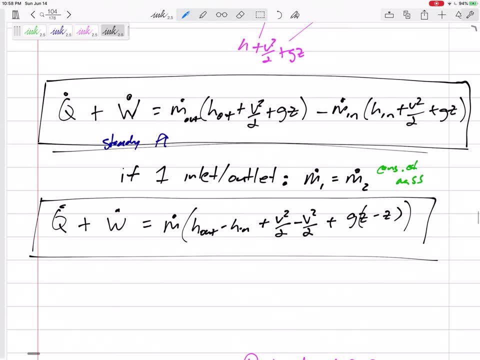 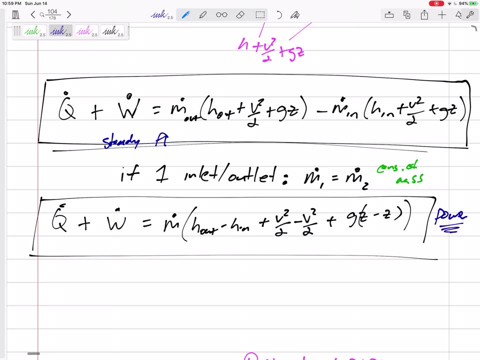 the kinetic energy together, the enthalpy together, if we want to. So. so here's an equation. We could write that down. but again, it's really this, this first equation, that top equation: This was a power, This was power. right, Q, dot, W, dot. We had. 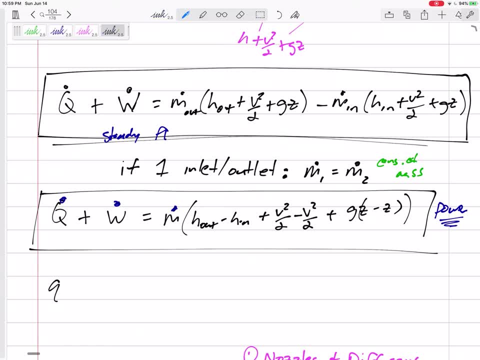 M dot. Uh, what about lowercase? What about specific? The difference between power and specific would just be: we get rid of this M dot. It would just be: Delta H, Delta K, E, Delta P, E. So so this you know. here's another equation. This is the specific equation. 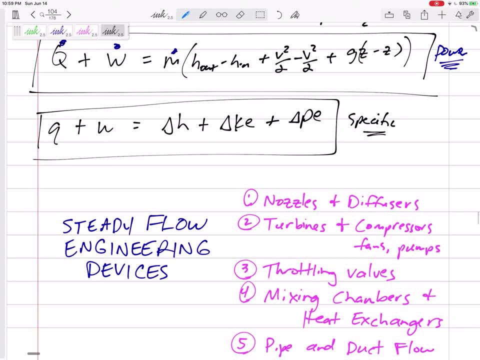 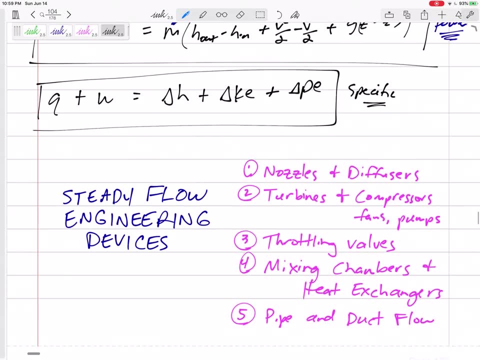 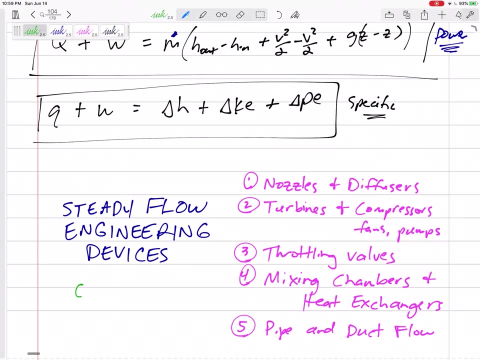 Okay, So for steady flow device like nozzles, diffusers, turbines and compressors and pumps, throttling valves, mixing chambers and heat exchangers and pipe and duct flow, we can. so this is what I'm going to do: We can start. 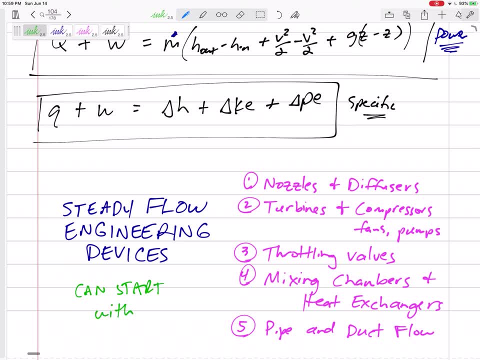 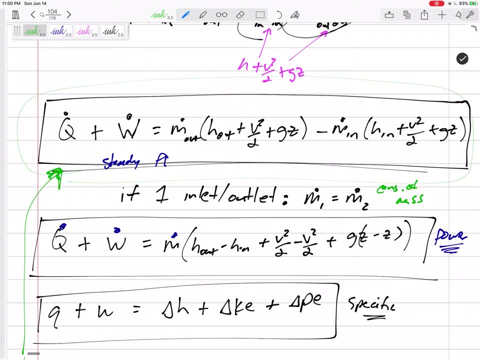 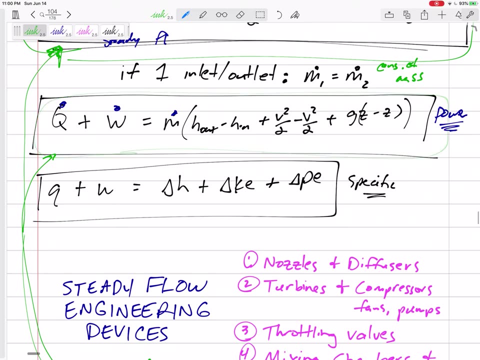 with. I like to start up here. right, I like to start up here. but if we know there's one inlet and outlet, then we can go right here. If we know there's one inlet and outlet and we only want specific, we can go right there. 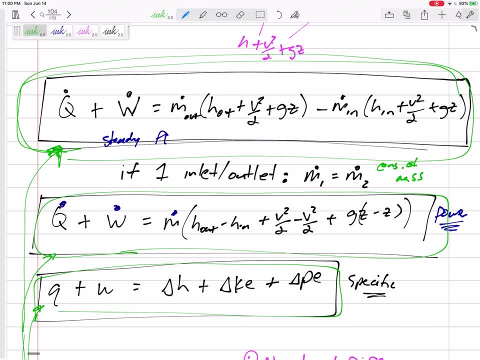 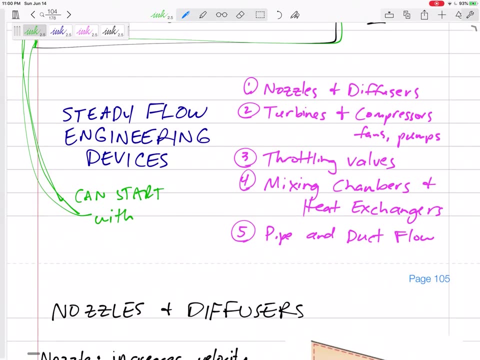 But in general I'm, I'm going to start with this top one, our main equation, Um and and and we've got that equation, So maybe we take that equation. We solve for some unknown right, We solve for some unknown, and don't forget. So can start with these, uh. 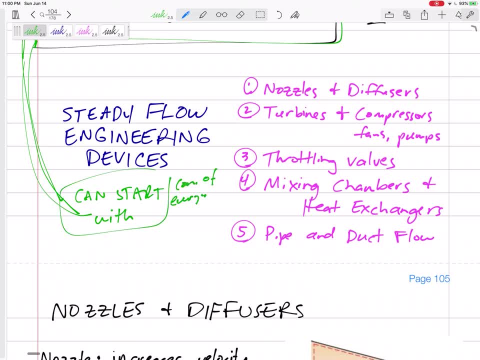 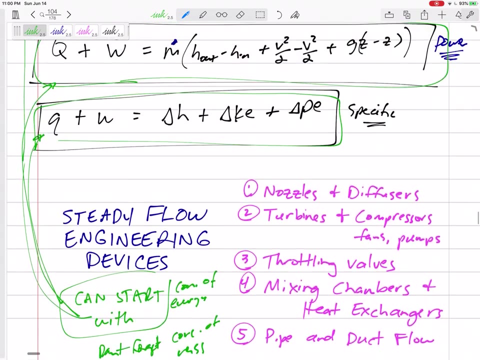 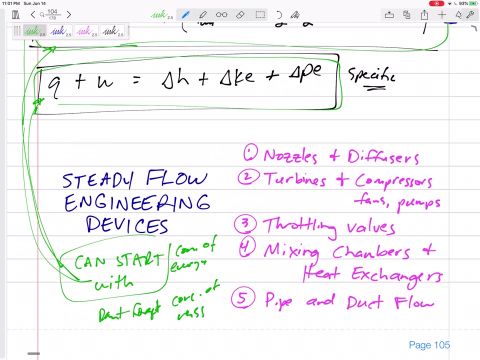 energy, conservation of energy, don't forget conservation of mass. If there's not one inlet and outlet, then we might need to really think about this min and mout. Um, if we've got two inlets and one outlet, the two inlets have to equal the one outlet, right? 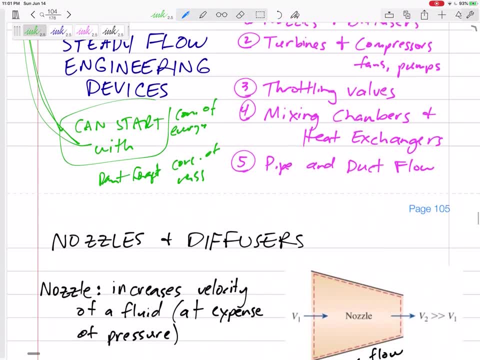 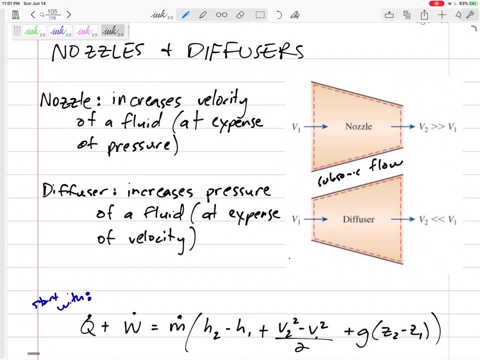 Okay, So let's talk about some of these nozzles And diffusers, turbines and compressors, startling valves, talk about these different types of steady flow devices. So so what I'm going to do, I'm just going to give you, in general, this is usually how we'll handle a nozzle and diffuser. you know, in general, this is how we're going to handle compressors and turbines in general. 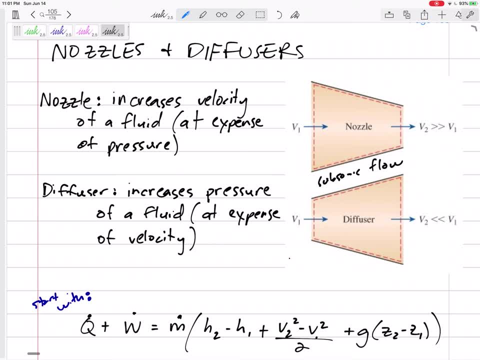 Now, you know, the problem might be a little bit different, but these are just generally how they're. they work. nozzles and diffusers either increase the velocity or decrease velocity. right Nozzle increases the velocity, a diffuser: 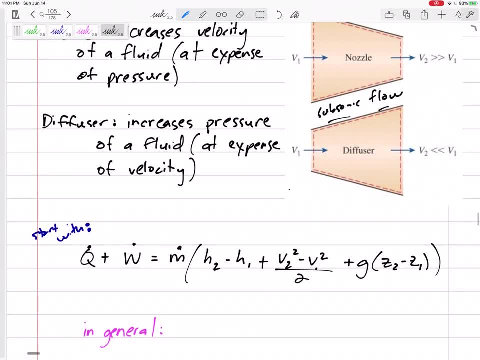 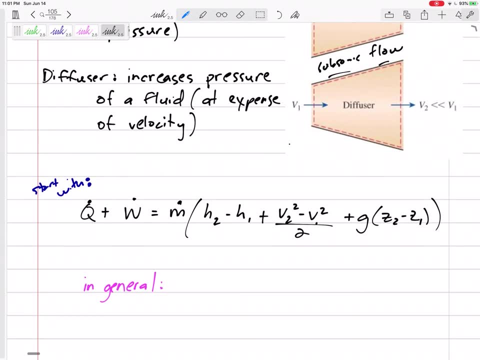 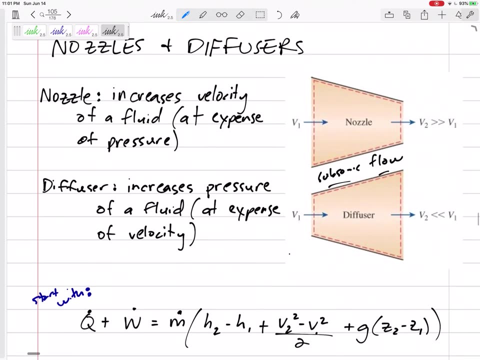 Decreases the velocity, uh, if we're in subsonic flow, uh, by changing the cross-sectional area. if we start with, Q plus W equals mdot, right, because this is one inlet and one outlet, um and and a. a a diffuser is just a backwards nozzle, right? 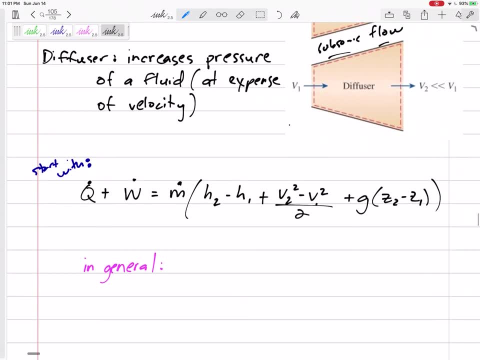 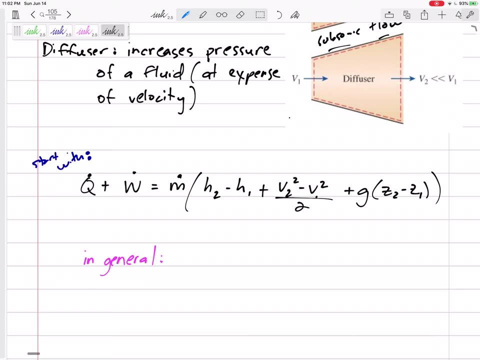 You just just flip the the same uh device. So in general we start with: Q plus W equals mdot, delta H, delta K. Uh, in general there's probably not going to be any change in height from inlet outlet to inlet. 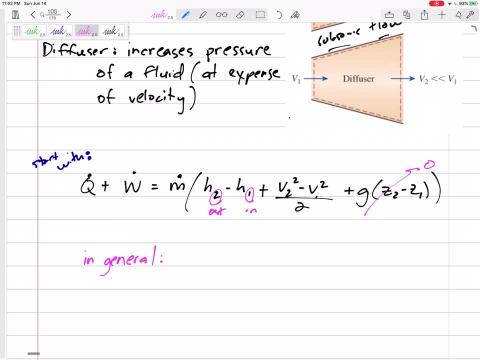 Here. two is outlet, one is inlet, Two is outlet. one is inlet. Two is outlet, one is inlet. Don't get it confused with like initial and final. This is outlet and inlet. In general, there's no potential energy. 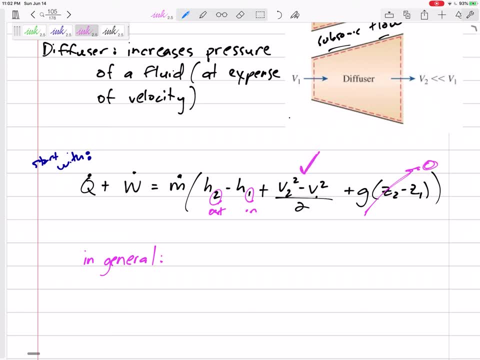 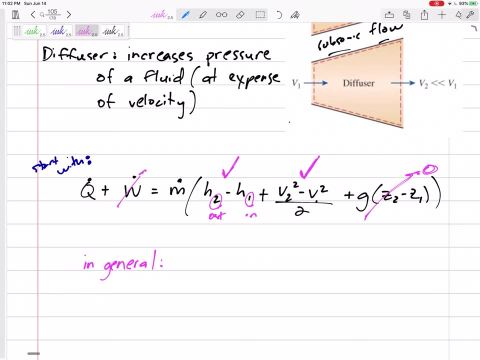 There is usually velocity change in velocity. That's kind of the whole point of these nozzles and diffusers. So we will have that. We will definitely have H? Um, in general we're not getting work out or putting work in. 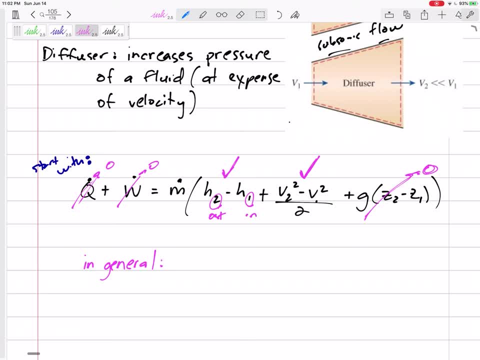 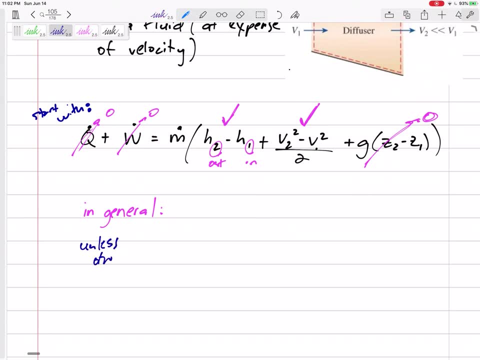 In general, we're not losing heat or putting heat in, you know, unless they tell you So, unless otherwise told. unless otherwise told, nozzles and diffusers: Qdot equals zero, Wdot equals zero, potential energy equals zero. 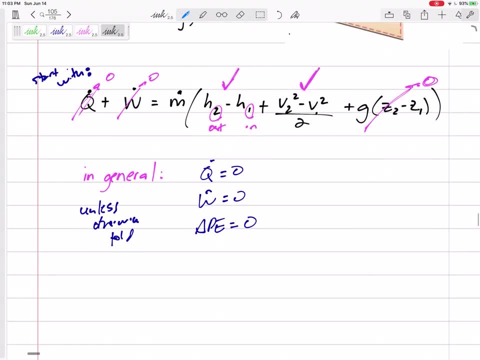 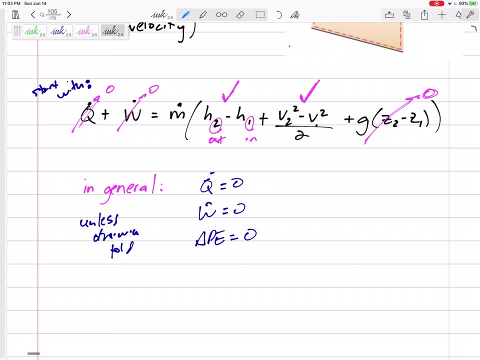 And so we're left with What We're left with. zero on the left-hand side equals Mdot H2 minus H1 plus V squared 2 minus V1 squared over 2.. If this is zero on the left-hand side, I can divide the Mdot out over also. 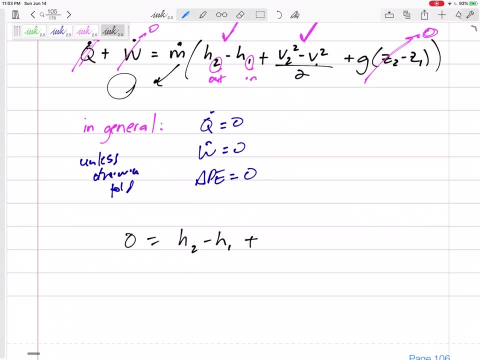 And so I can say H2 minus H1, V squared 2 minus V1 squared over, And so I can say H2 minus H1, V squared 2 minus V1 squared over 2, equals zero. So you know that that works. you know, 75% of the time for nozzles and diffusers. 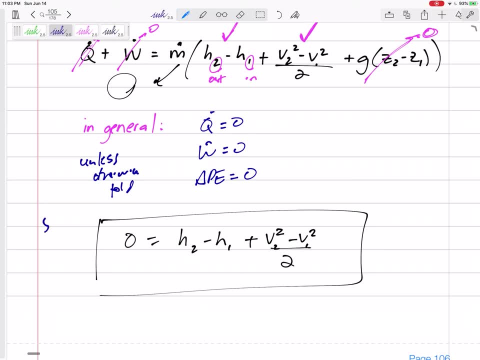 If you want to write that down, you can you know on your, on your formula sheet. But this is for steady flow. This is for a nozzle or diffuser, with no Q or W. Um, I like to start with this. 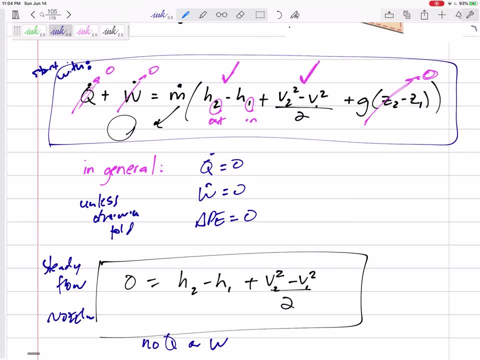 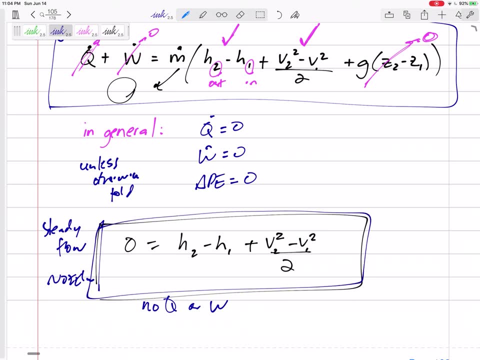 I like to start every problem with that. If it's one, if it's steady flow, one inlet, one outlet, and then things go to zero. But in general, here's our what we do with a nozzle or diffuser. 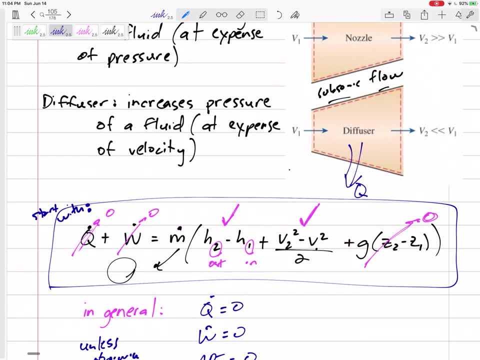 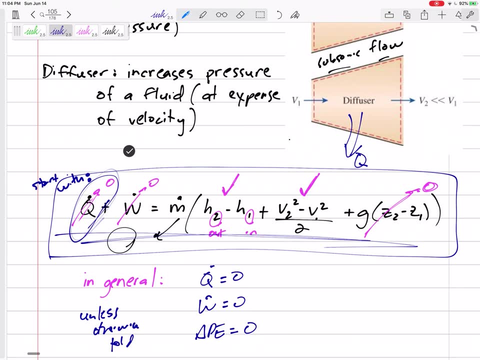 What if we had a diffuser and it said something about some Q going out? Then we would need to to start with this And we would need to to plug in whatever Q value it told us for that one. Okay. Turbines and compressors. 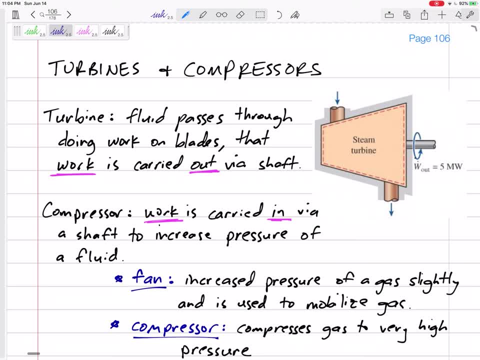 Um, A turbine gets work out by fluid going through it. You can think about, you know, putting a uh like a, a dam like a in a stream. Um, The fluid going through there can turn the blades can turn a shaft. 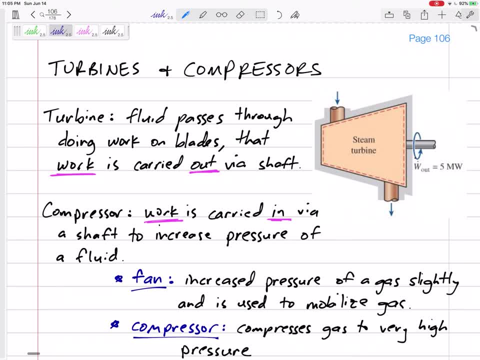 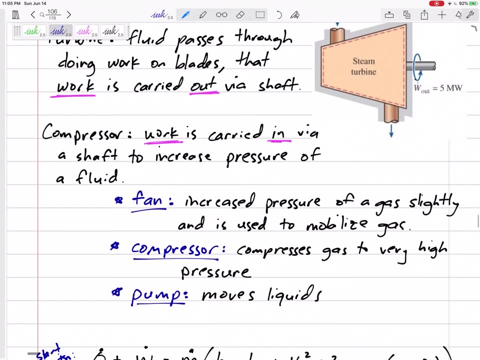 We can get work out of a turbine. A compressor is backwards. We put work in in order to push Blades that will push the fluid out. So for turbines, work is carried out via the shaft. for a compressor, work is carried in uh via the shaft. 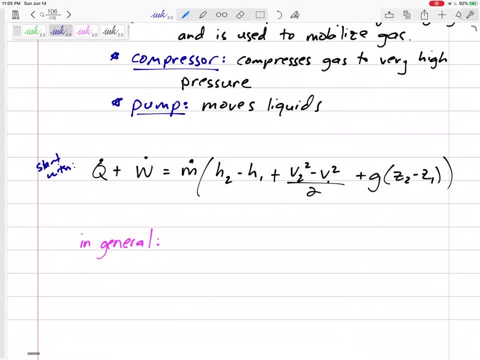 Uh, but it's the same device, just worked, just plugged in backwards. So we're starting with this because it's one inlet and one outlet. It's steady flow: one inlet, one outlet. We can start with this one in general, in general, 75% of the time. 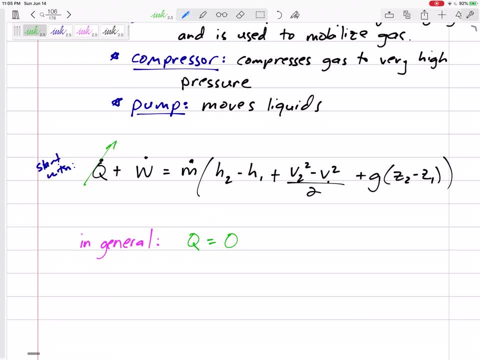 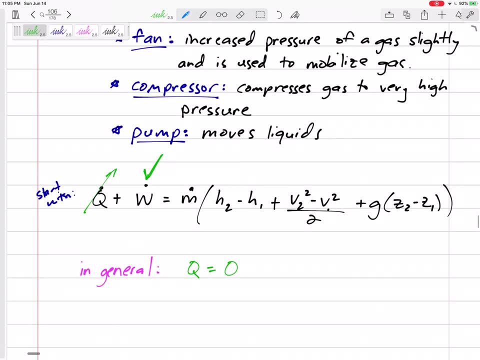 It works all the time. There's no Q, There definitely is W. That's the whole point of a turbine is to get the work out. And for compressor you definitely have to put the work in. Um, there's depth, There's always going to be H for all these city flow. uh, device problems. 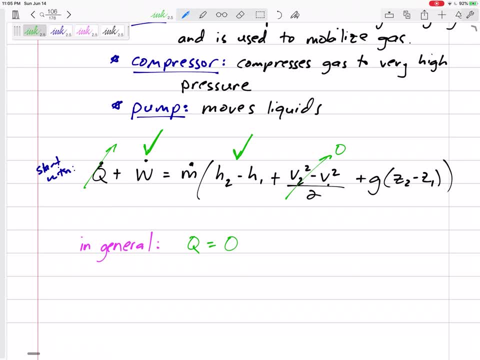 If it doesn't tell you. in general it doesn't really increase or decrease the fluid going through there, At least not very much, And probably doesn't change the height unless we're told So. So in general the change in the kinetic energy is zero. change of potential energy is zero usually. 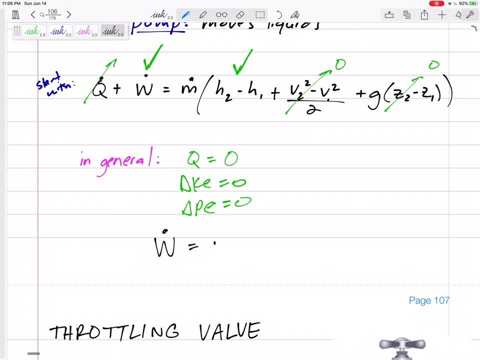 So usually the work is M dot H two minus H one. in general, the work, the power is M dot H two minus H one. So a few things, a few things to think about. two is always outlet, one is always inlet, whether we're. 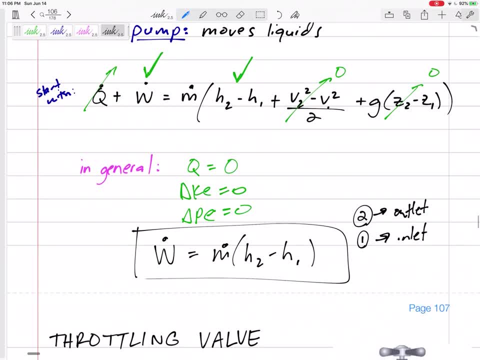 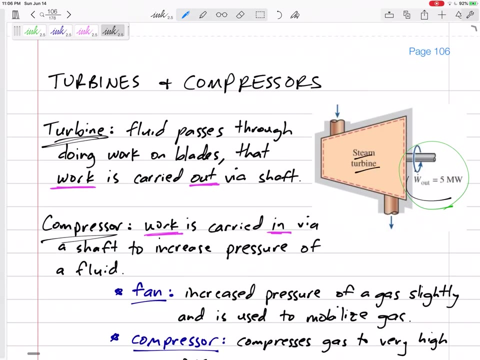 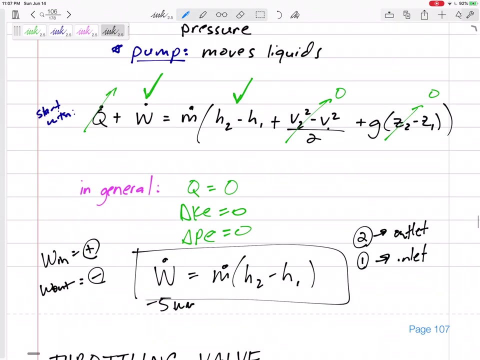 we are looking at a turbine or a compressor and remember how I do these: work in is positive, work out is negative. So this right here, if this was a steam turbine, this work coming out, I would plug in negative five. you know it'd be negative. five megawatts on left-hand side equals. 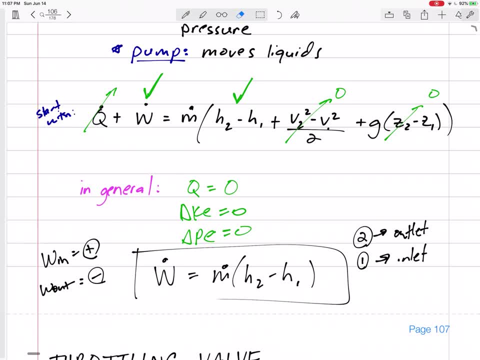 And so I could, you know, figure out that Delta H right there, All right. So remember, twos are outlets, ones are inlets, uh, and work in is positive, work out is negative, The way that I define. that's why I've got Q plus W. the book might do it opposite. 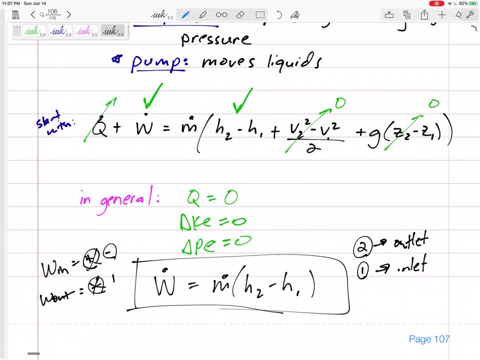 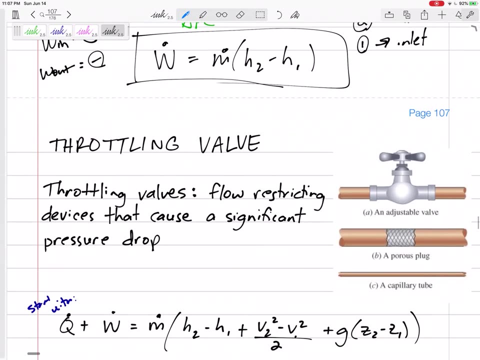 They'd say Q minus W, and they would. they would put minus and plus. but you see how we would both work out to the same answer. I'm putting Q plus W and I'm saying: work in is positive, work out is negative. Okay, 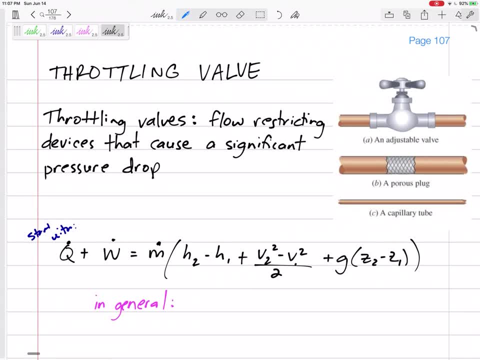 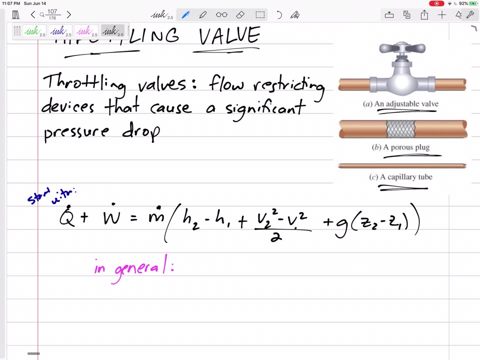 Uh, a throttling valve is a flow restricting device. Uh, it can be called a capillary tube, a porous plug, an adjustable valve or a throttling valve. Um, it restricts the flow and it causes a significant pressure drop. 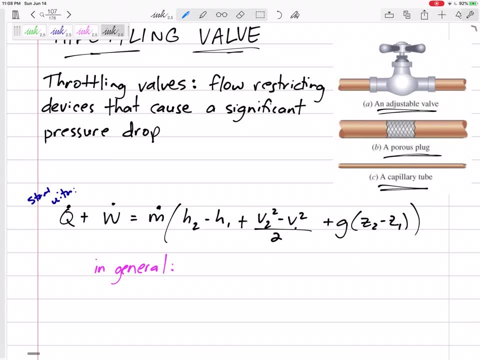 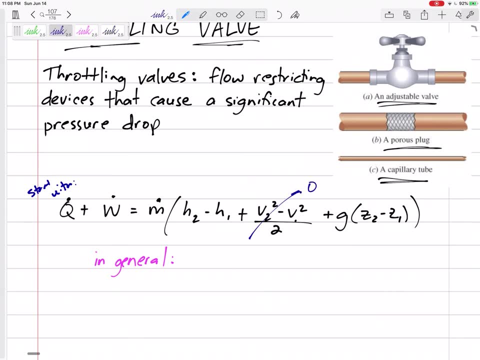 That's kind of the whole idea of a throttling valve is to drop the pressure. drop the pressure. The idea of throttling valve is actually negative: Not to change the velocity, not to change the height, and actually it. it takes no work. 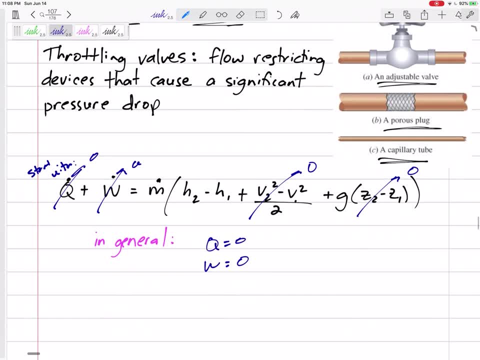 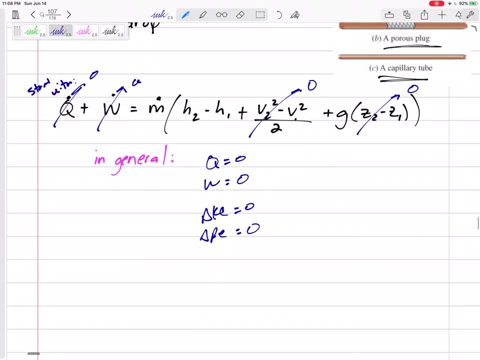 Uh, and in general they are adiabatic. So in general the Q is zero, the W is zero. the change in kinetic energy, everything is zero. for throttling valves The whole key is: throttling valves are constant infelpy process. 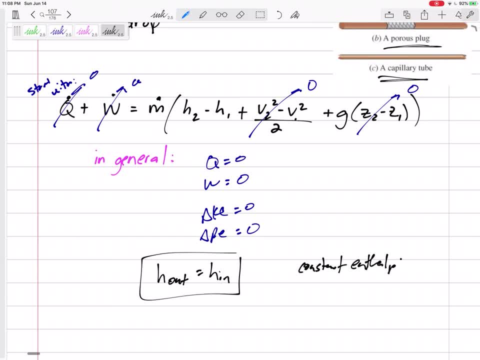 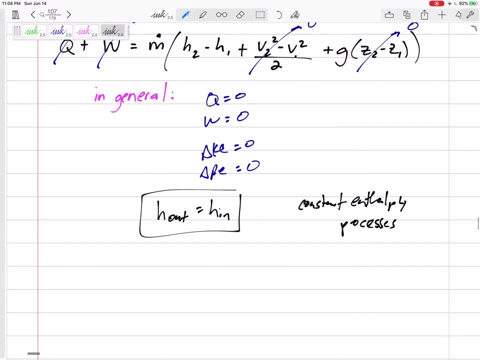 Constant Enthalpy processes. All right, So H out is equal to H. and how? how I mean? why would that help us? Why would we even use that? Well, H is U plus PV. So we can kind of expand that and say the U out, pressure out V out. 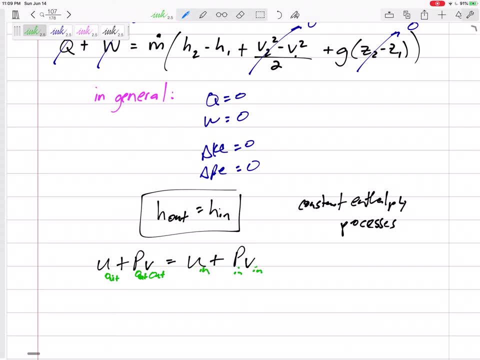 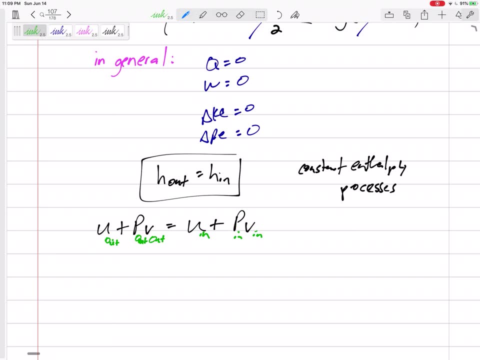 Uh, the, The outlet equals the U in, pressure in V in, And so if, if we know a few of these, we can find another, if we know a few of these, we can find another. one more thing before we move off of this one for an ideal gas. 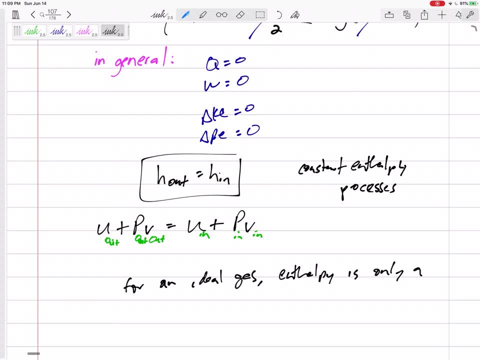 Enthalpy is usually only a function of temperature, only a function. Okay, Dim, Oczywiście am. I am using a. There is an equation for what? Poinzium of temperature. and so if antibiotica is constant, uh, temperature is constant. if enthalpy is constant, temperature is constant. Okay. 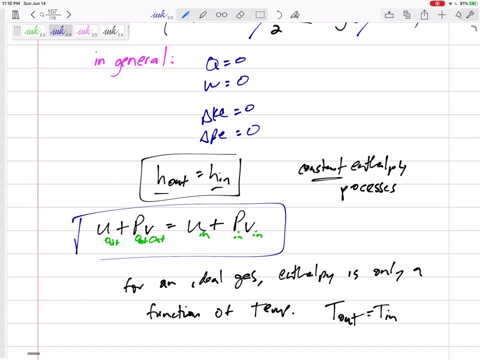 but so, So right. here is really our equation. There might us-. 4- Throttling valves, Also called capillary tubes, porous plugs. Enthalpy of the inlet is equal to the enthalpy of the outlet, and the u plus pv of the inlet equals u plus pv of the outlet. 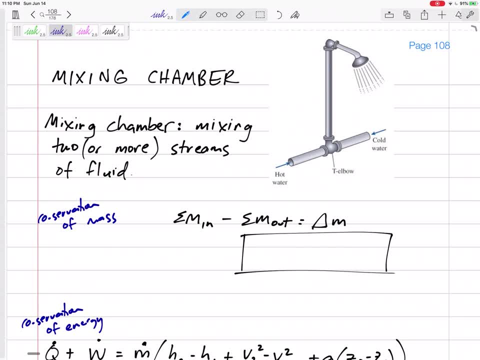 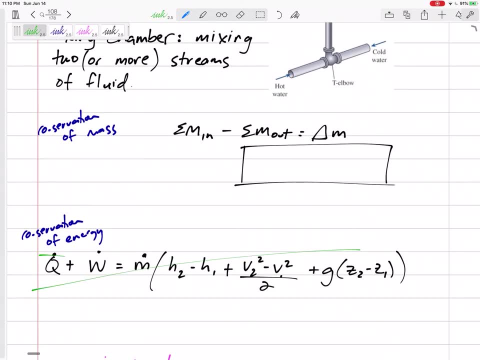 Alright, how about a mixing chamber, A mixing of two or more streams of fluid? Now with this one, with this one. we cannot start with this equation. did you notice this equation? we had factored the m dot out, saying that m dot inlet was equal to the m dot outlet. 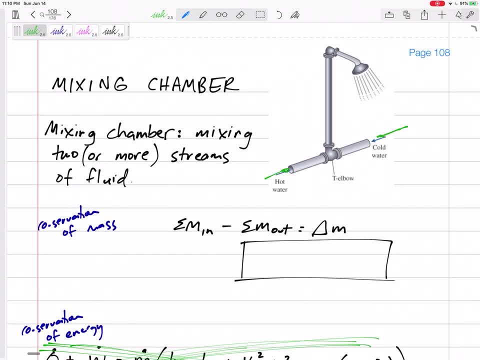 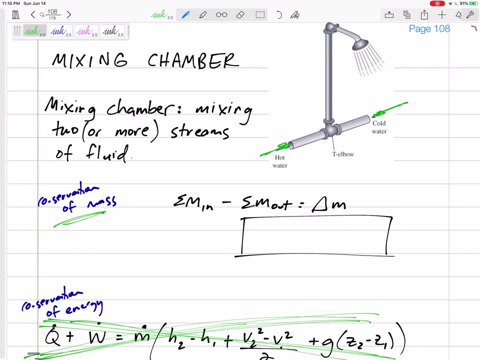 but here we might have two inlets, two separate inlets, right here. So alright, we're going to need our conservation of mass equation. if this is a steady flow device, there's no change in mass. The sigma m in equals sigma m out. 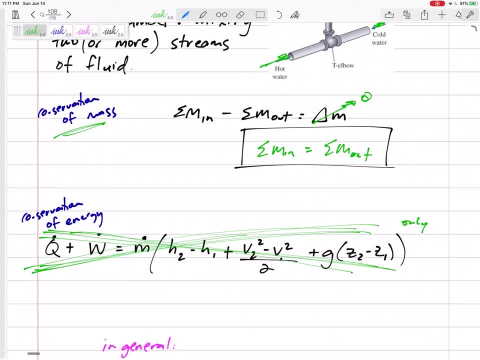 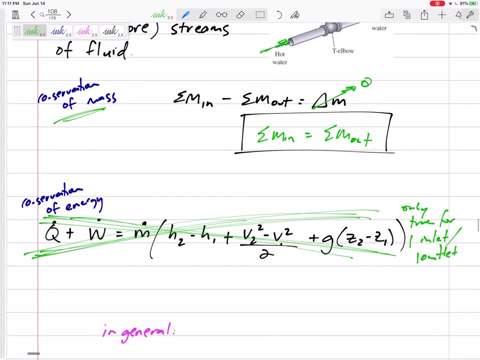 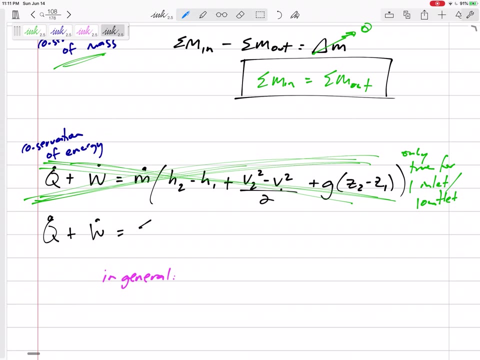 to m dot out. Alright, This was only true for one inlet, one outlet. Alright, we've got to go back and start with this equation: Q plus W equals summation of all the m dot outs, H plus V squared over two plus G Z. 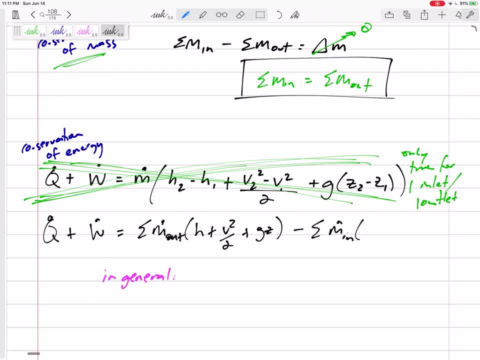 minus m, dot in time, each one's H plus V squared over 2, plus GZ. So there is the equation that we need to start with for a mixing chamber. Now, in general, W is 0, Q. all right, heat transfer. 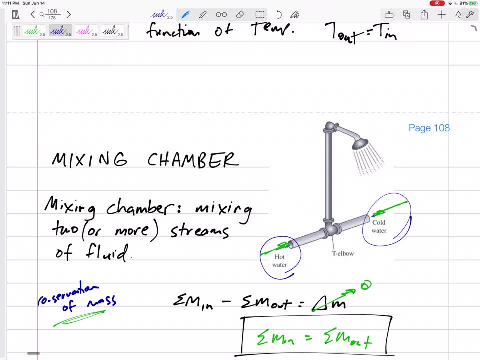 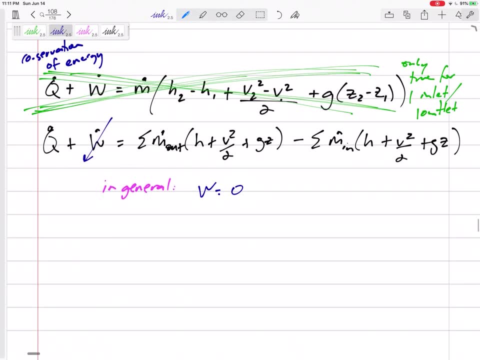 It seems to me like heat transfer is a big part of this. We've got cold water and hot water coming out to make warm water. Isn't there a heat transfer? There is a heat transfer, but it is internal, Internal When we're looking at this whole conservation of energy, of the whole system, 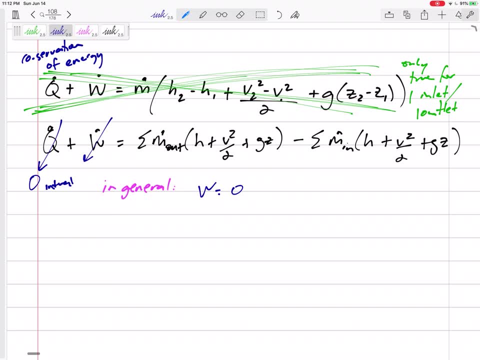 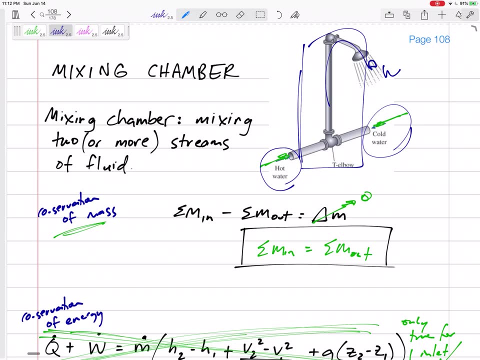 yes, there's heat transfer back and forth between hot and cold, but if the hot and cold are both part of our system, then there's no Q. In general there's no Q, It is internal. Now, unless it tells us there's some Q going out, 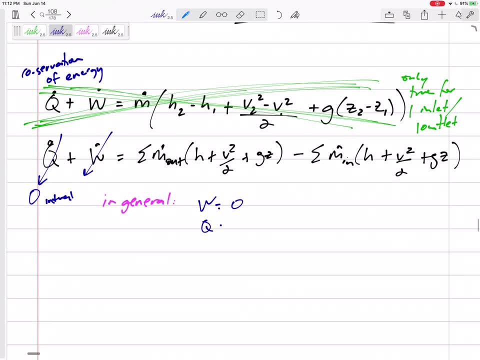 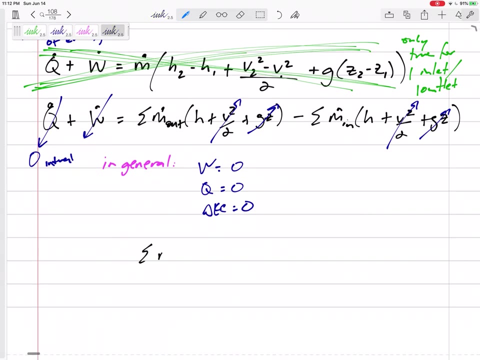 but in general the Q is 0.. Kinetic energy is 0.. So don't worry about kinetics, Don't worry about potential energy. Do you see what this really boils down to? The M dot out, H out equals the M dot in H in. 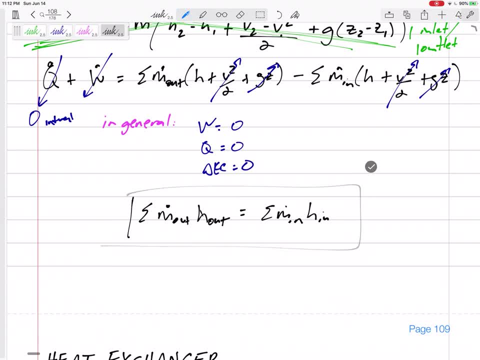 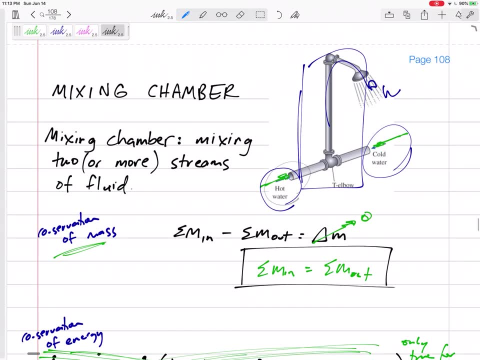 There we go. So that is our equation in general for a, for a mixing chamber. So I'd take the M? dot of the hot time, the H of the hot right. So so for instance, I'd say M? dot, hot, H, hot. 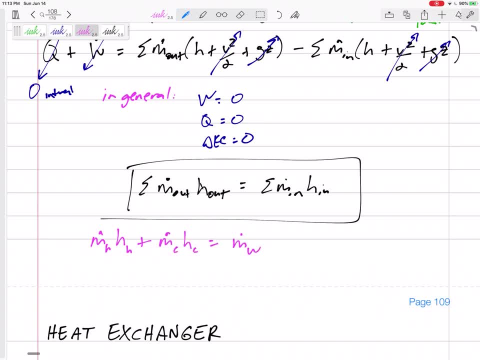 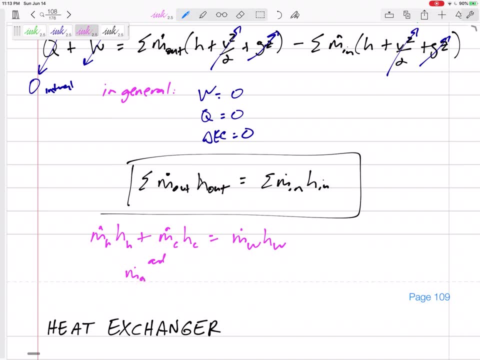 M dot cold- H cold equals M dot warm, H warm right. So there's one equation and M dot, that's conservation of energy. conservation of energy, But we also have conservation of of mass: M dot H plus M dot cold equals M dot warm. 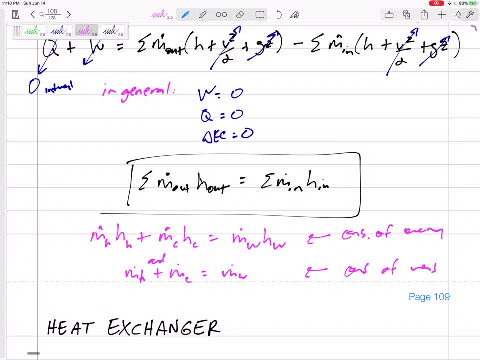 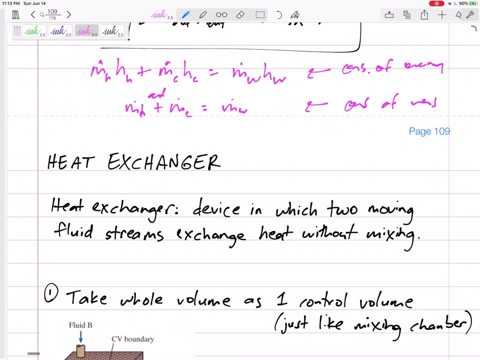 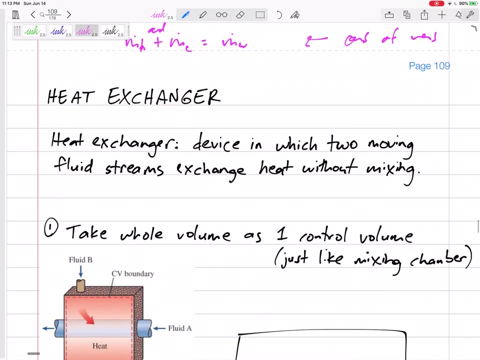 So two equations that might help us plug in and solve. Okay, Last, I think last one. No, not quite, Not quite. Two more, two more, heat exchanger. Heat exchanger is just like a mixing chamber, except they don't really mix the fluid streams: exchange heat without mixing. 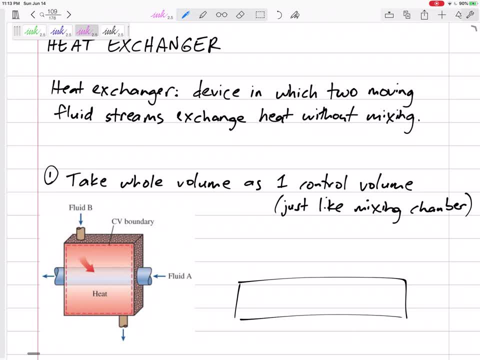 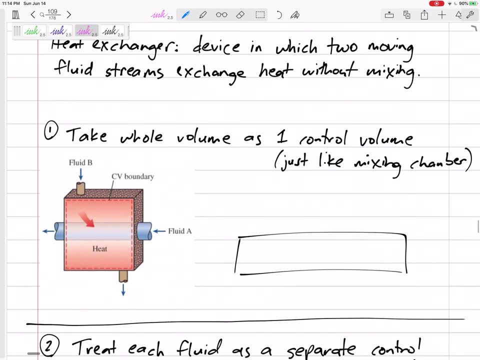 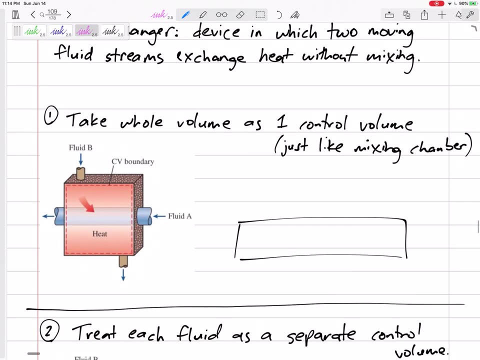 All right, We have two methods for looking at heat exchangers. We have two methods for looking at heat exchangers. Method one is to treat the whole volume as one, or method two is to treat each fluid separately. All right, If we treat the whole volume as one. 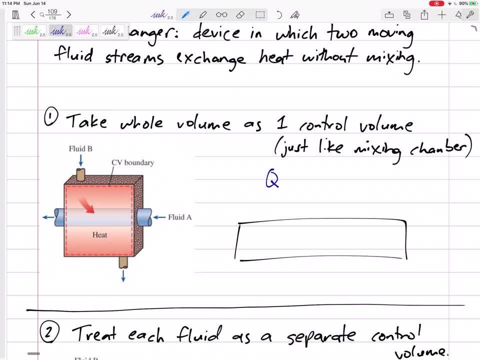 it's just like a mixing chamber. The heat transfer is internal, The heat transfer for is internal, so it is zero and it's it's just what we got: m dot out, h out equals summation of m dot n, h, n. so that might be an equation to use that might be helpful for us to use like for so so 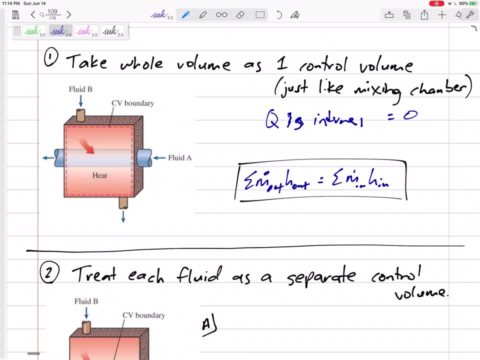 for instance, let's say we have so for a heat exchanger, we've got a fluid a that's coming in and a is going out. b is coming in and b is going out. so it's like we have two inlets right here and we have two outlets. so you know, we might have like the m dot a. 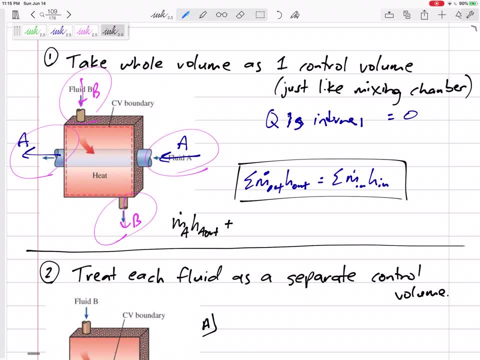 h a out m dot b h b out equals m dot a h a n. m dot b h b n. you see that, you see how that we would do that if we have two inlets and two outlets, there's no, no need to do conservation of mass, because a doesn't exchange with b, so there's. 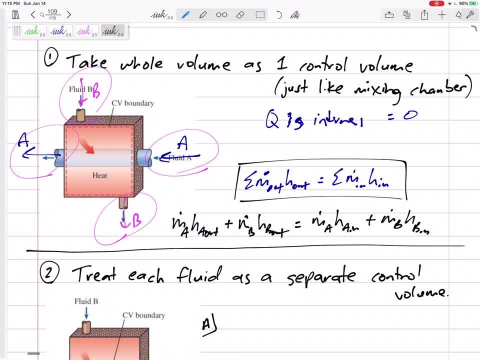 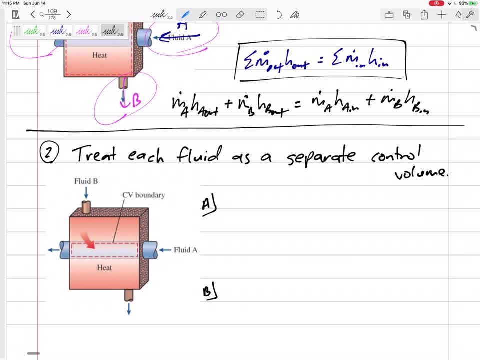 only the m dot of a is just m dot of a, it's not m dot of a different for the inlet and the outlet. all right, but if we treat them separately, so if we only look at a, only look at a, then we do have some q coming in and it'd be something along the lines of this: 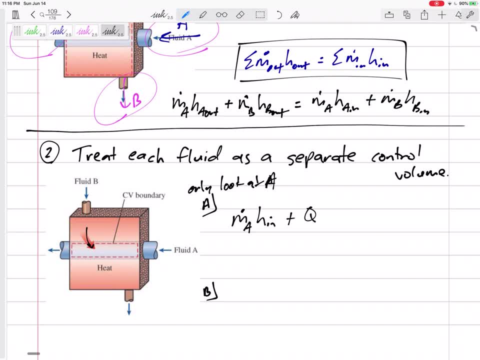 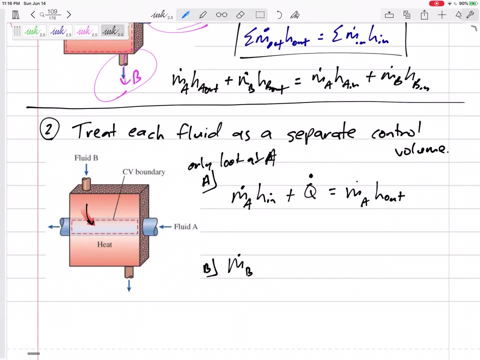 m dot a- h n plus the q between the two equals m dot a- h a out or m dot b, so b is the hot fluid. the heat transfer is going from the hot to the cold. m dot b- h of b in minus the q that it's leaving equals m dot b- h b out. this is the same q, same. 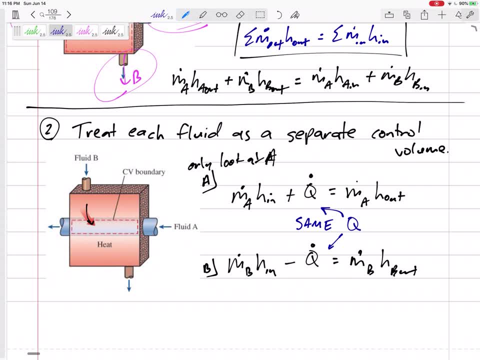 value for q right here and here, right. doesn't that make sense? i think that makes sense. if you're only looking at a, then it's just going in and going out and it's getting some q in to it. if you're looking at B, then it's M dot H going in, M dot H going out, and it's. 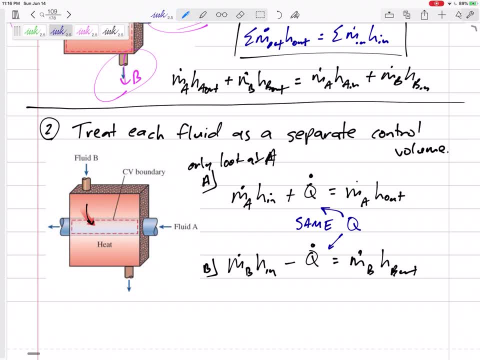 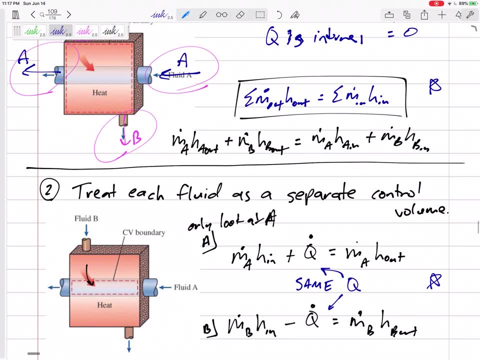 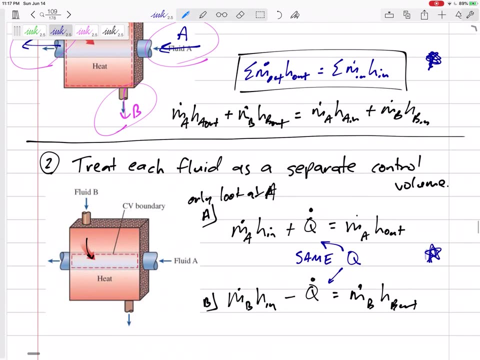 losing Q. It's losing Q. You might have to do both of these methods in order to solve for what we need. Might have to do both of these methods to solve for what we need. Alright, and lastly and easiest, because I'm just going to say: 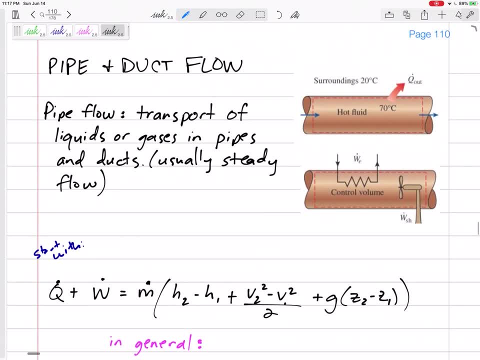 this is pipe and duct flow transport of liquids and gases in pipes. Usually this is a steady flow. Usually there's not mass that's building up in the pipes. It might have work crossing the boundary. It might have Q crossing the boundary. The 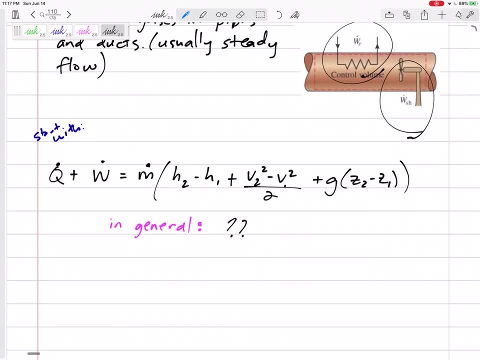 velocities might matter In general. I'm just going to say it depends on the situation. It depends on the situation And you know, all of these actually depend on the situation, And so my advice for you is to take this equation right here.